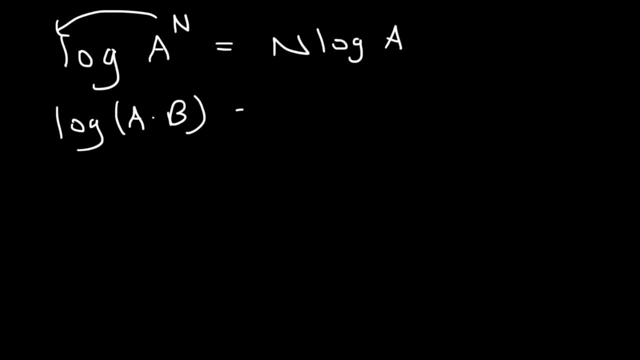 And log a times b. you can expand it as log a plus log b, And log a divided by b is going to be log a minus log b. Now, because a is on the top, it's going to have a positive sign next to it. 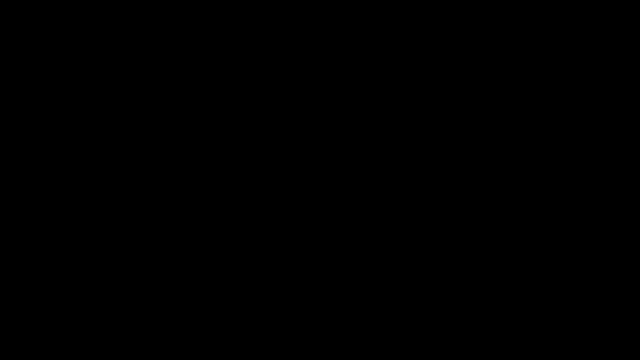 b is on the bottom, so it has a negative sign next to it. So consider this problem: Log x, y divided by z. Go ahead and expand the expression. x and y are both, So it's going to be positive log x plus log y. 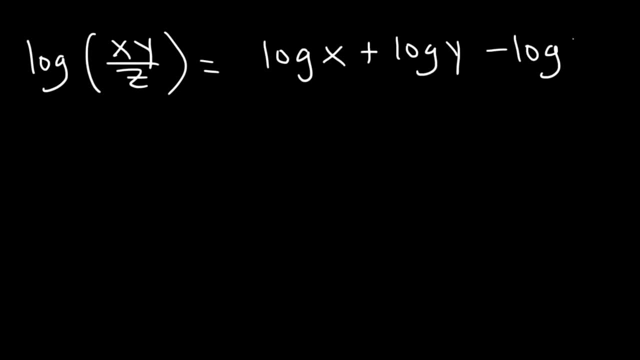 z is on the bottom, so it's going to be minus log z. Try this one. Log a squared b to the third, c to the fourth, d to the fifth. Go ahead and expand it. So a and b are both on top, so it's going to be positive. 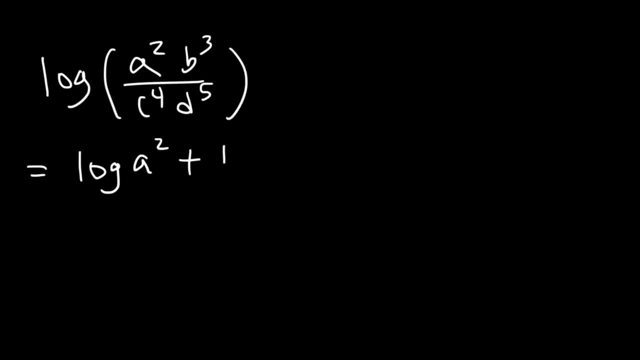 Log a squared plus log b to the third. c and d are on the bottom, so it's going to have a negative sign in front of it. So it's going to be minus log c to the fourth, minus log d to the fifth. 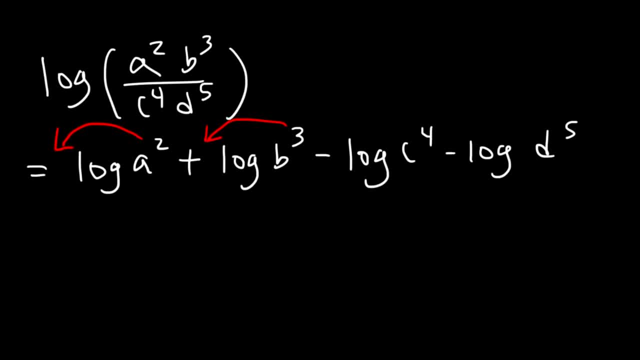 Next, we need to move the exponents to the front, And that's the last thing that we need to do. So the final answer is: 2 log a plus 3 log b, minus 4 log c, minus 5 log d. 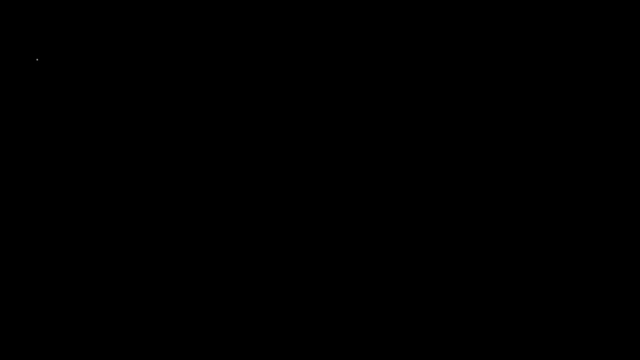 And that's it for this problem. Let's try one more example. Go ahead and expand the log. Let's say, if it's the square root of a times b to the one-fourth, divided by the cube root of c to the fifth, raised to the third power, 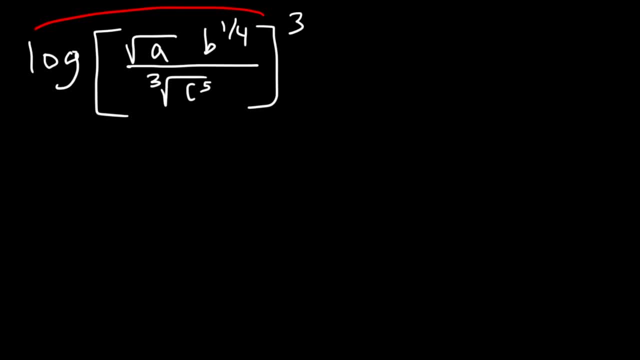 Now the first thing that I would do is move the 3 to the front. So this is going to be 3 log, And then next we need to get rid of the radicals. We need to write them as an exponential fraction. The square root of a is basically a to the one-half. 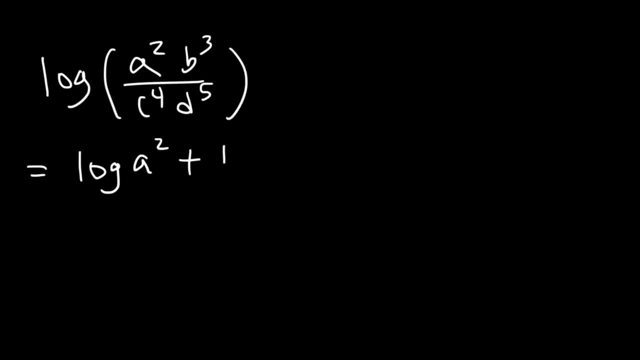 Log a squared plus log b to the third. c and d are on the bottom, so it's going to have a negative sign in front of it. So it's going to be minus log c to the fourth, minus log d to the fifth. 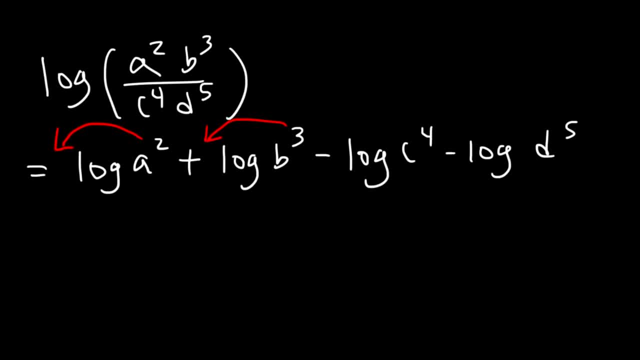 Next, we need to move the exponents to the front, And that's the last thing that we need to do. So the final answer is: 2 log a plus 3 log b, minus 4 log c, minus 5 log d. 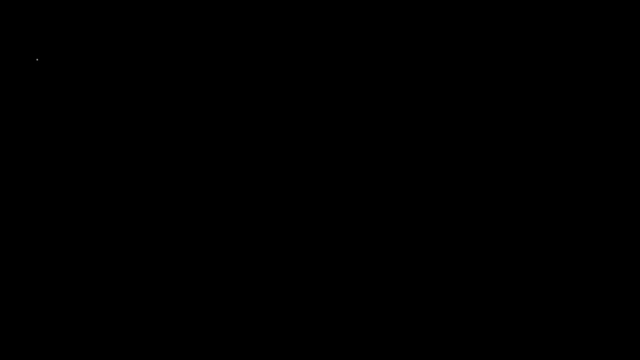 And that's it for this problem. Let's try one more example. Go ahead and expand the log. Let's say, if it's the square root of a times b to the one-fourth, divided by the cube root of c to the fifth, raised to the third power, 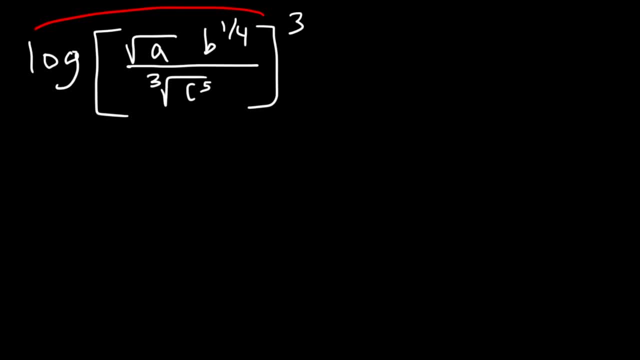 Now the first thing that I would do is move the 3 to the front. So this is going to be 3 log, And then next we need to get rid of the radicals. We need to write them as an exponential fraction. The square root of a is basically a to the one-half. 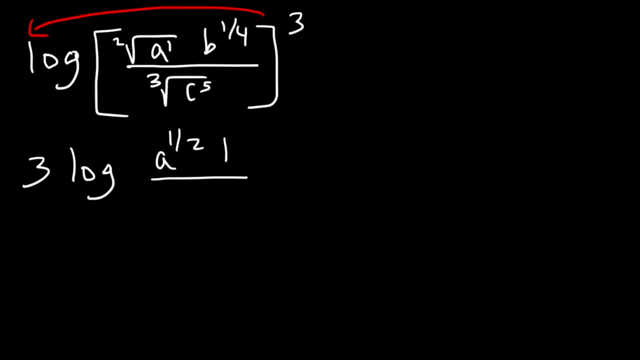 The index numbers are 2.. And then we have b to the one-fourth. The cube root of c to the fifth is basically c raised to the 5 over 3.. So now we can expand it. So a is on top. 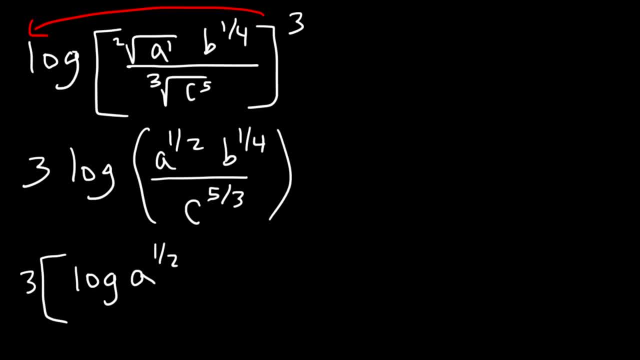 And so is b. So it's going to be positive log a to the half, plus log b to the one-fourth. Now c is on the bottom, so it's going to be minus log c to the 5 over 3.. Now let's move the exponents. 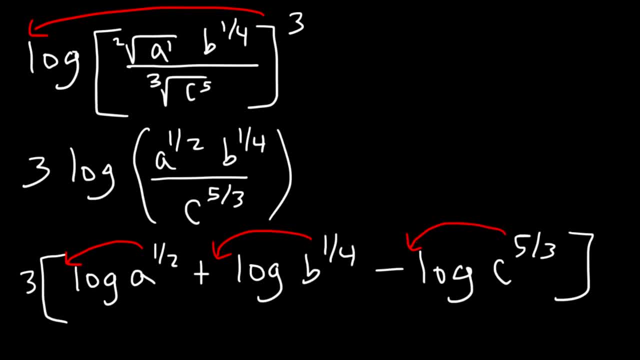 Let's move the exponents to the front. So we're going to have 3 times one-half log a, plus one-fourth log b, minus 5 over 3 log c. Now the last thing that we need to do is Distribute the 3..